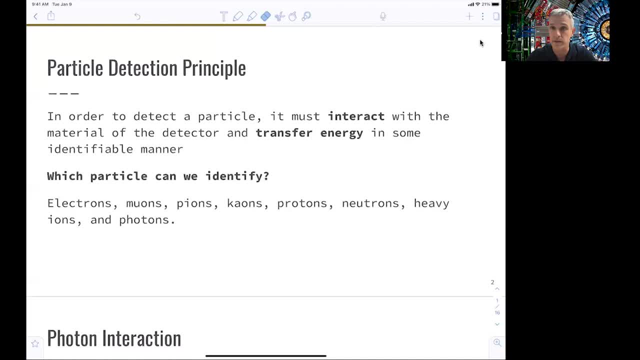 decays before it has a chance to interact with the detector. The same for a top quark, a Higgs photon and so on. Interesting neutrinos. Neutrinos interact with the detector very, very rarely. When they do, the actual detected signal is not of the neutrino directly, but of the 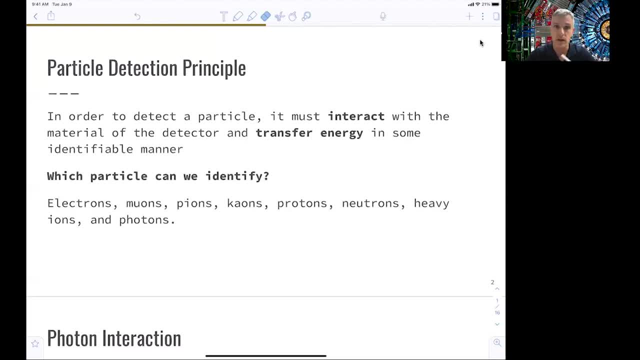 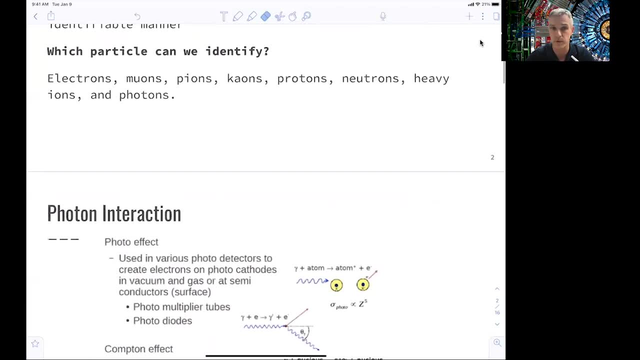 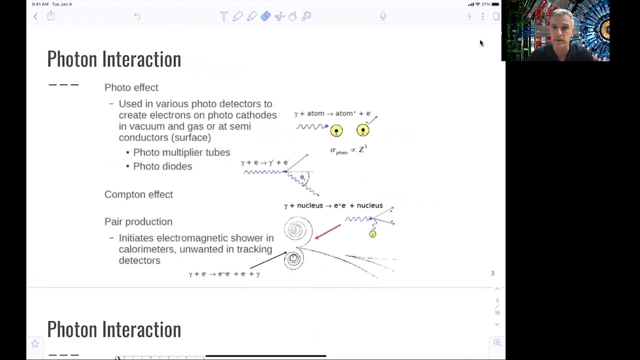 products of the interaction. So we will split this discussion up in the interaction of neutral particles and charged particles and we start with a photon. So the photon interacts with detector material, with material in general, via three leading effects: The photo effect, Compton scattering and pair production. 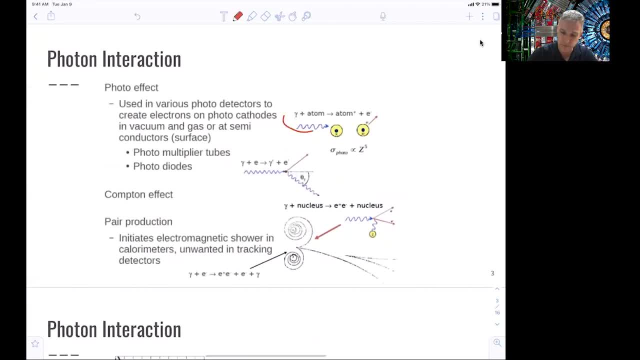 In the photo effect we have a photon interacting with an atom and then kicking out an electron, And then your detector has a chance to identify the energy and the momentum of the electron. This concept is used in photomultiplier tubes, where then the electron? 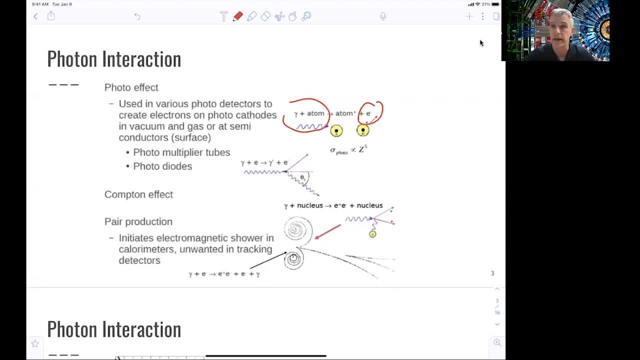 the kicked out electron is further amplified And that leads to a shower of electrons which can be measured. All the photodiodes use this effect. We have discussed the Compton effect quite a bit Here. the energy of the scattered electron can be. 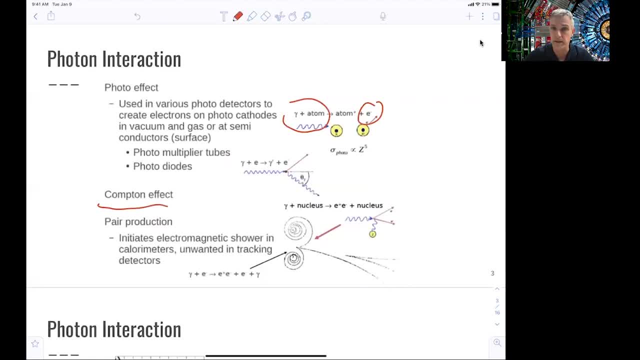 measured also the energy of the scattered photon. And then there's pair production. Pair production dominated high energies, And it typically is part of an initiation process of electromagnetic showers in calorimeters. That's great. So what happens in the calorimeter? 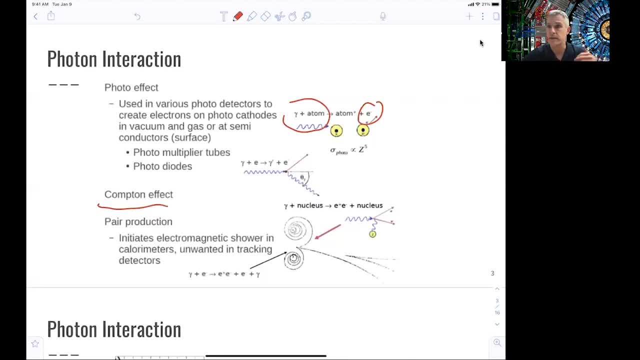 and we'll talk about this more later- is that an incoming photon or electron causes this photon to convert into pairs of electrons and positrons, And then there's this cascade of electrons and positrons and additional photon being produced In tracking detectors. this is unwanted, So therefore build tracking detectors rather thin. You don't want to have this. 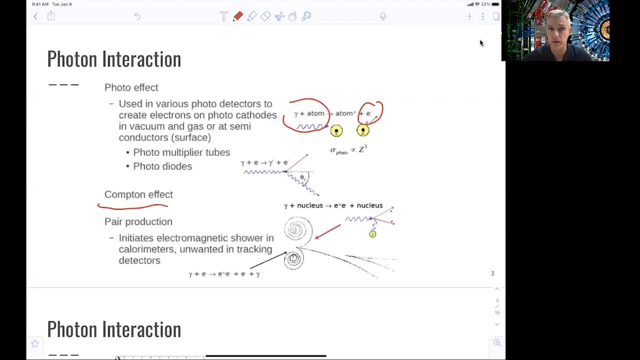 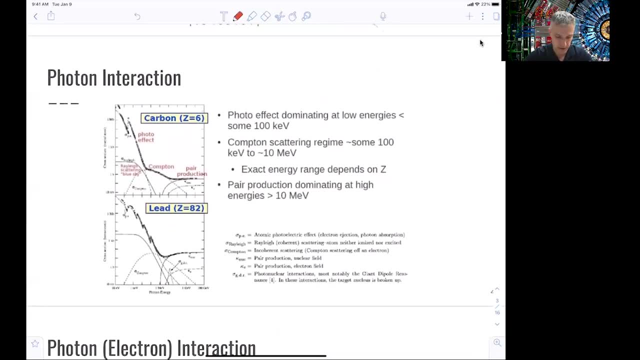 confusion of additional charged particles And we try to measure the energy of the photon. So this plot here shows you the cross-section as a function of the photon energy And you see here very nicely those three effects contributing to the total cross-section. So for low energies, 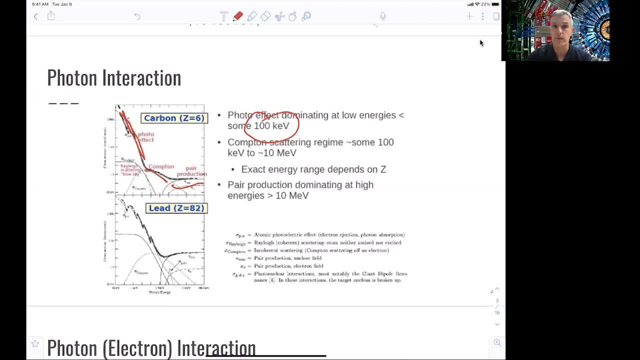 in the range of some 100 keV the photo effect dominates. Then there is this intermediate range from about 100 keV to about 10 MeV, where we see the effect of Compton scattering, And every thing above this is dominated by pair production, And this here shows you that there are some. 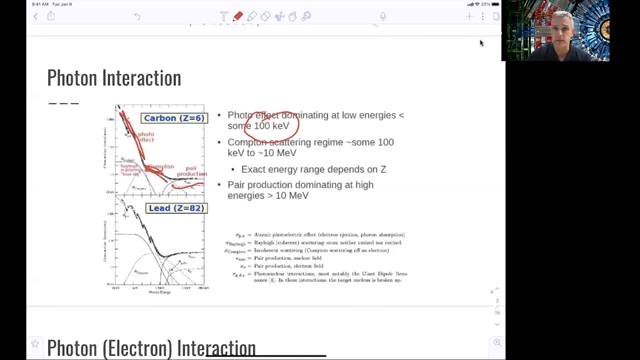 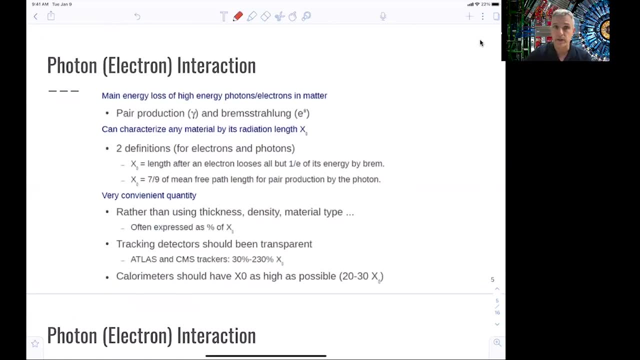 differences in what kind of material you interact, of course Photon or electron interaction Again. so the main energy loss mechanism for high energy photons and electrons in matter is through pair production and also Premst-Strahlung. Premst-Strahlung is the effect when electron or positron radiates a photon. 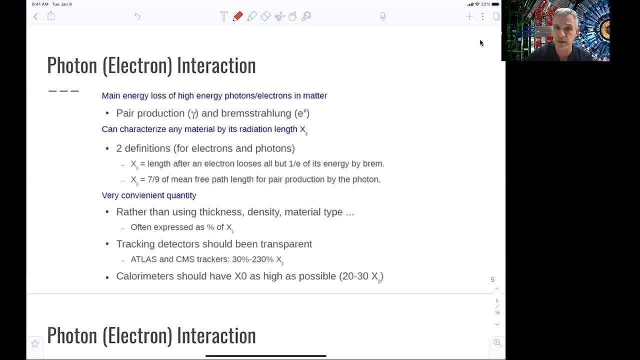 You know, you can characterize the materials by introducing a concept of radiation length, And there's some confusion sometimes in the definition. They're very similar but they're not quite the same. Radiation lengths can be defined as the length after which an electron 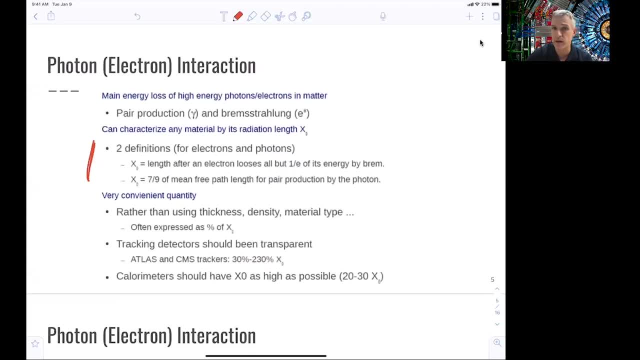 loses about 1 over e of its energy by Premst-Strahlung And you often find the definitions through the mean free path length And x0, the radiation length is defined as 7 nines of the mean free path length. 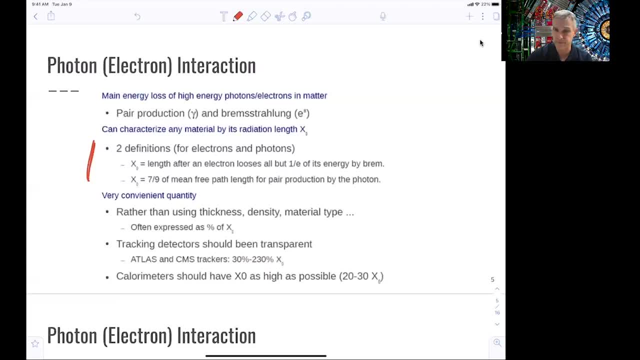 So those are the two definitions and they're typically used in the regime where the process is dominant. It's a very convenient property or quantity because you don't have to worry about when you, when you're thinking about the interaction of the detector, about the specific thickness and what it means. 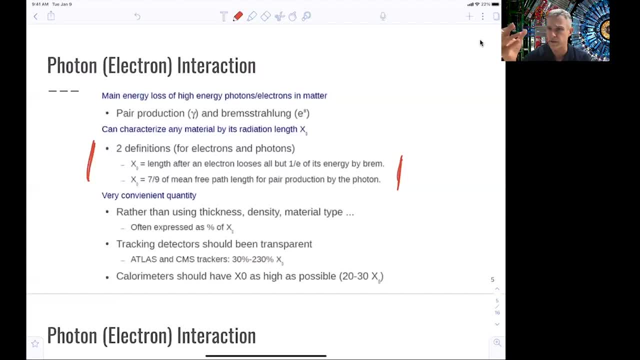 in terms of energy loss And simply know that. you know your piece of lead is a fraction of the energy loss that's being generated by the electron. So that's where we have the problem of a radiation length And that tells you how many of your photons. 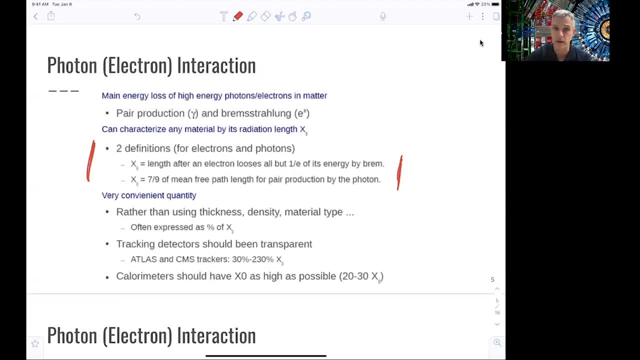 actually or how much of the photon energy is being lost. Typically, when you build detector concepts like a collider experiment like ATLAS or CMS, you want the tracking volume to be of low radiation lengths And for ATLAS and CMS this depends on the rapidity. 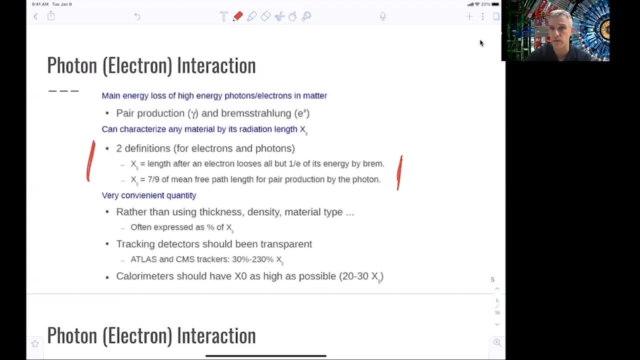 or the forward direction, But it varies between 30% and 200% of a radiation length. And for calorimeters you want that all the energy is deposited in the calorimeter and nothing is leaked out in the back, And therefore you design calorimeters typically. 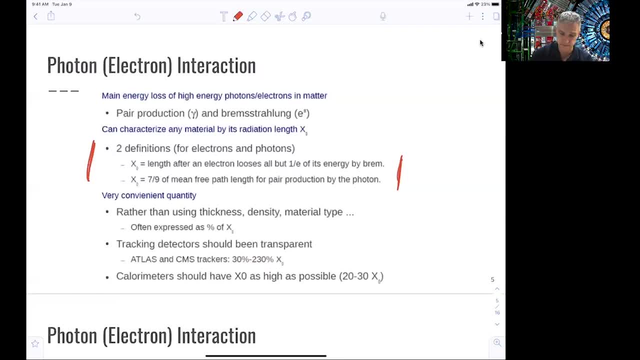 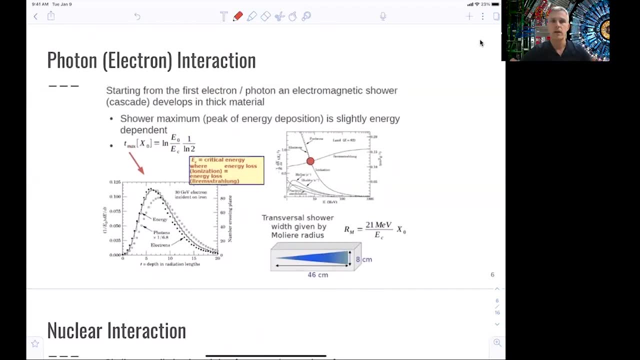 with 20% or 30% radiation length in mind. So again, when we think about how a photon or an electron leaves a footprint in a calorimeter, you start from this: first The first electron and photon, And then this particle evolves in an electromagnetic shower. 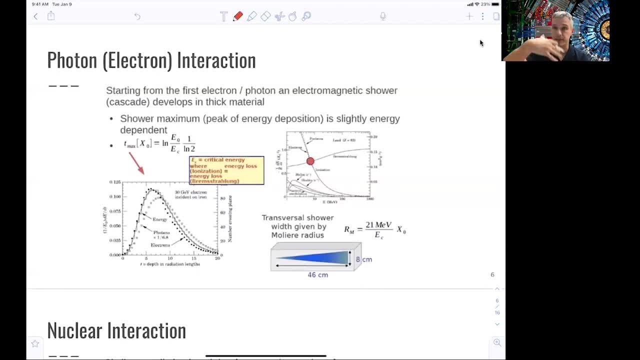 So there's this cascade effect as the particle tries to move through this material. The shower maximum is given here Slightly depends on the energy. It sees this logarithmic dependency. I introduce here the critical energies. This is where the energy loss through ionization. 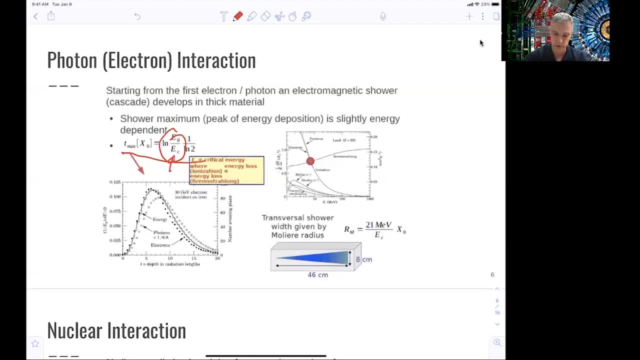 is equal to the Brems-Schwallen And you see this in this plot. here It's rather small as a function of energy. the energy loss- Again you see this effect here- is from ionization And this effect here is from Brems-Schwallen. 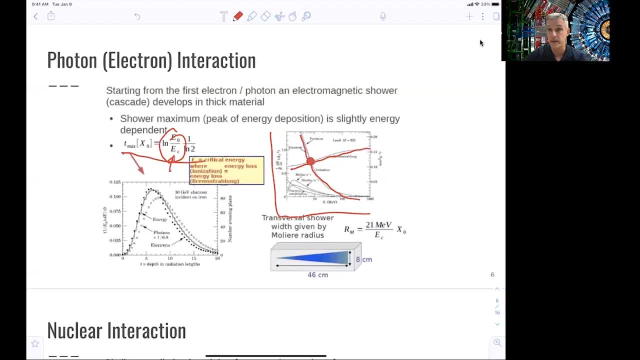 The critical energy is defined as where those two energy loss mechanisms give you the same result. So this is just a normalization factor. But you see that there is this logarithmic dependency of the energy loss. You can also wonder how wide a shower actually becomes. 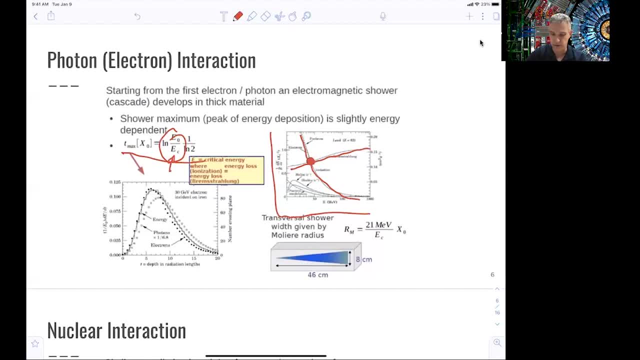 And this is given by the Brems-Schwallen, Given by the width of the transverse width of the shower, is given by the Moliere radius And that's approximate. You find 21 MeV over the critical energy times. the radiation 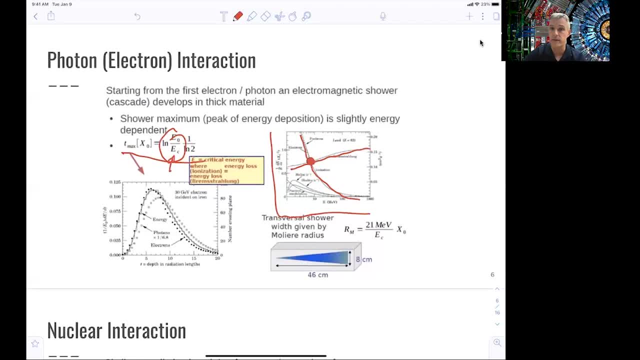 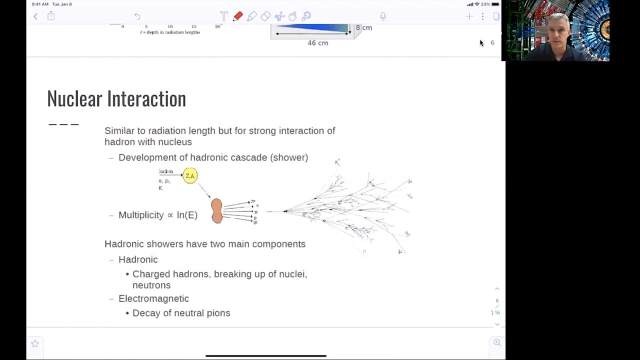 length gives you the size of the transverse size of your shower, And in this example this is 8 centimeter compared to the shower length of 46 centimeters. This is a very quick Summary of electromagnetic showers. You can also have nuclear showers, of course. 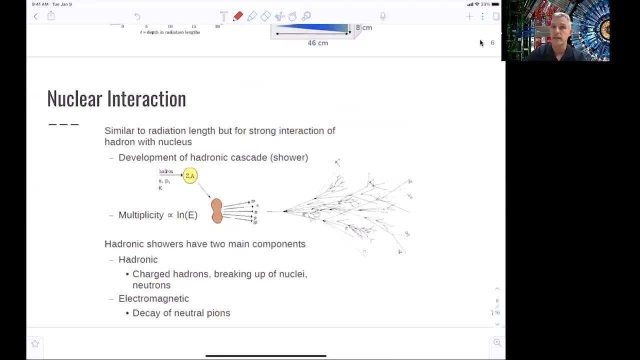 You have a neutron or a proton entering your calorimeter. Here the physics is a little bit more complicated, But you can introduce similar concepts. this concept of radiation lengths for strong interactions of the hadrons with the nuclei. So, as for the electromagnetic shower, 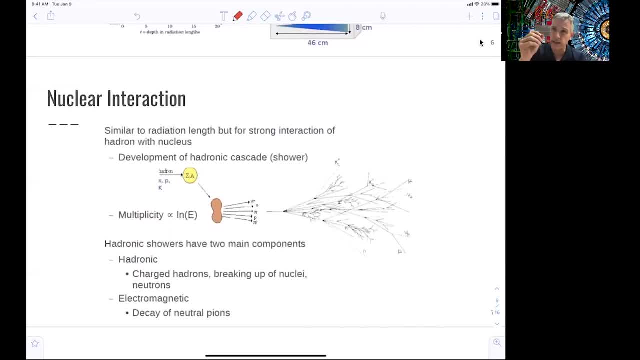 there is this cascade developing. However, if in the cascade, for example, you produce a neutron, that neutron can travel without leaving an interaction for quite a distance. So you don't have this continuous flow of energy, You have little clusters of energies. 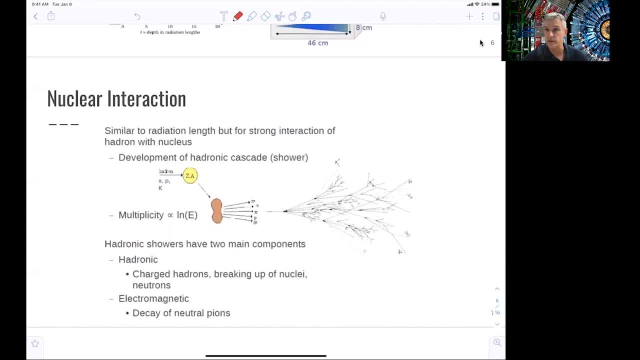 And in those clusters you have not just nuclear interaction but you can also produce new pions, And those new pions convert and decay into a pair of photons And then the photons they leave electromagnetic showers. So hydronic showers have typically two components. 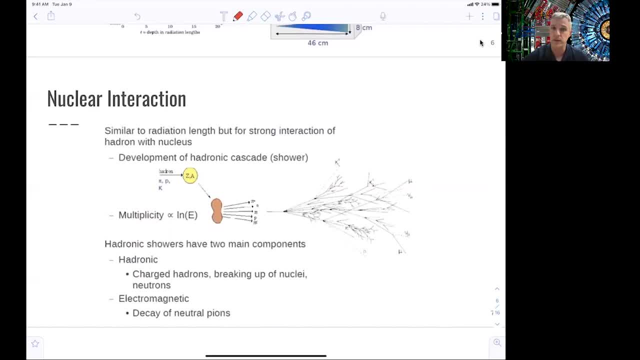 a hydronic part which is charged hadrons- You know, pions, kaons, protons, neutrons- and an electromagnetic part which is, as I said, coming from the decay of the neutrons or from the decay 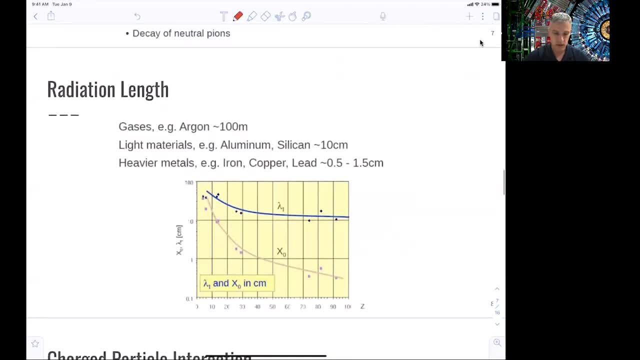 of the neutral pions, which are photons. So here, just to give you a feel for orders of magnitude, radiation lengths, given the nuclear and the electromagnetic radiation length given as a function of z, And for gases we are talking about hundreds of meters. 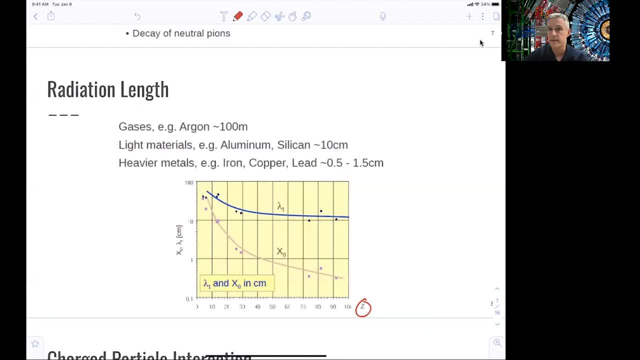 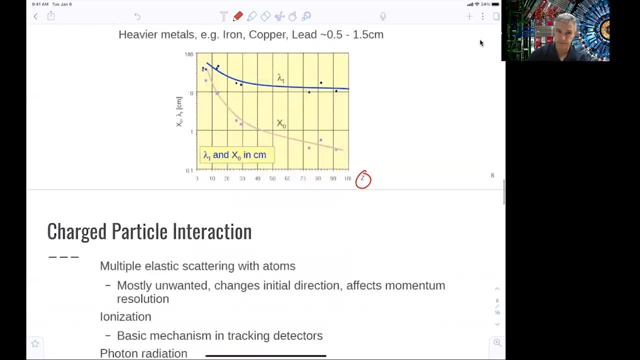 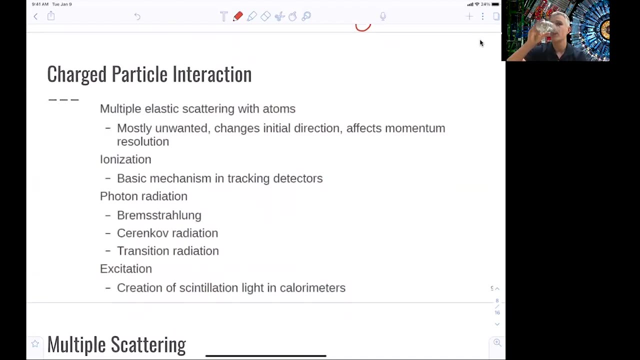 For light material- aluminum and silicon- we're talking about 10 centimeters, And for heavy materials, specifically lead, talking about subcentimeter radiation length. So moving from the neutral particles, from the photons and electrons, to the charged particle interactions. here again, just summarizing or giving 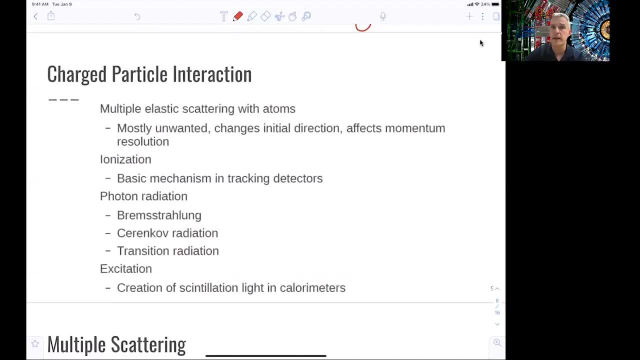 a summary first, and then going through the individual components. the interaction mechanisms are multiple scattering, elastic scattering with the atoms. This is a process which is not very much wanted, because when you try to monitor the trajectory of a particle, you don't want it to scatter and change randomly. 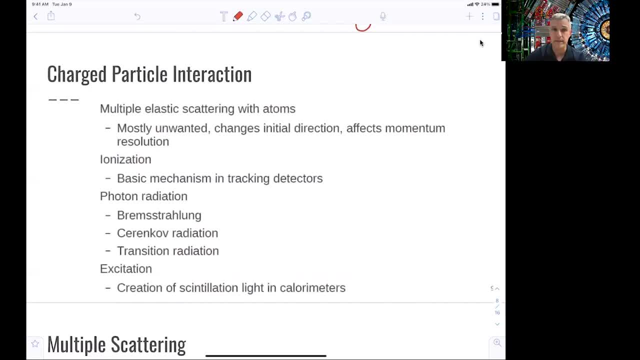 its direction or momentum. Ionization is a basic mechanism for tracking detectors. Photon radiation is an important part, through bremsstrahlung, but also through gerankophoresis Radiation or transition radiation, And then in scintillators you can excite the material. 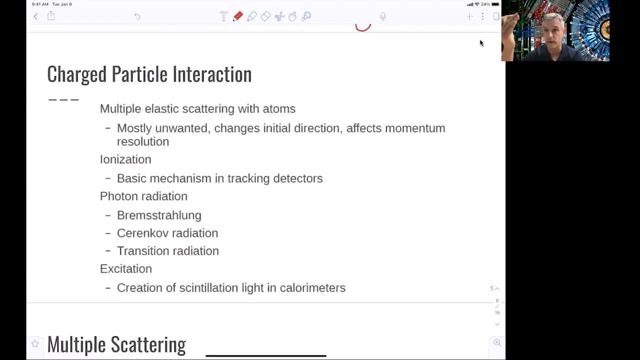 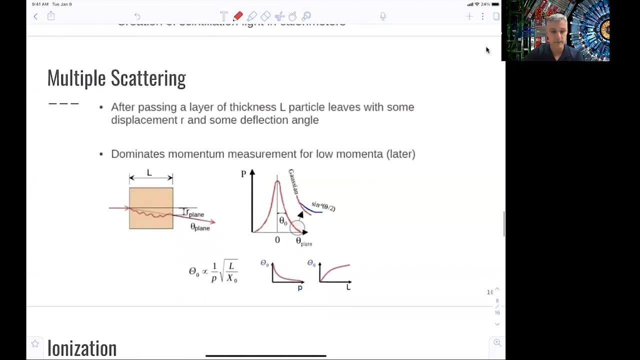 And then, if you have a wavelength-shifting material, you can cause scintillation light to be shifted in wavelength, And then you can read this out in order to gain information about particles going through. All right, let's start with multiple scattering. 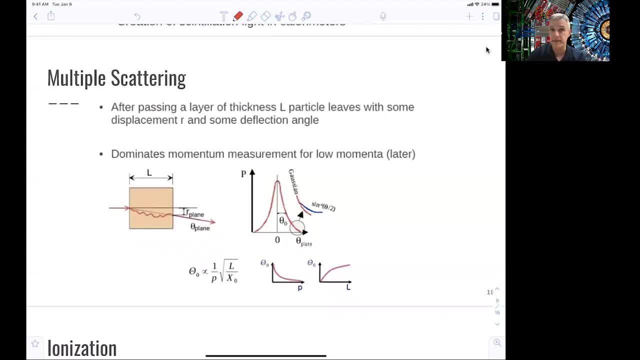 So after passing a layer of thickness with L, a particle leaves with some displacement, R And some angle of deflection. So that is problematic because you lose information through the random process And you see here this random Gaussian-like distribution which is rather annoying. 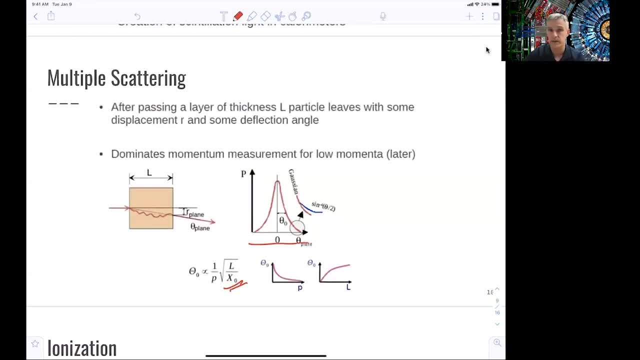 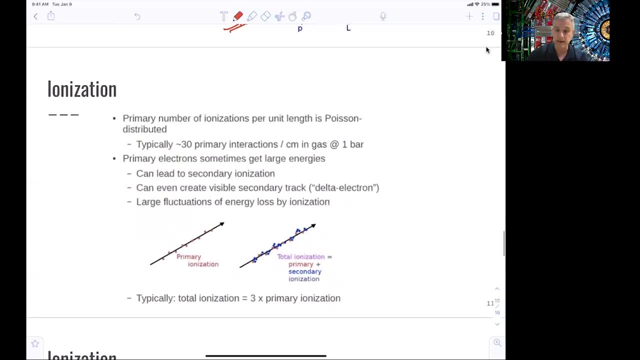 So the key here is to minimize the radiation length of the particle going through. Yeah, The next part is then on ionization. Again, this is the primary, The source of information we gain in tracking detectors. Typically, you have a number of primary interactions. 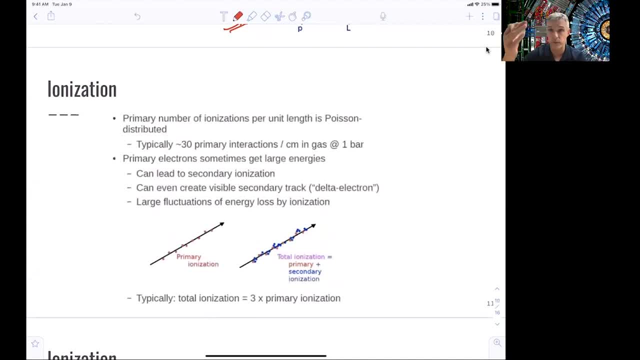 per unit length which are Poisson distribution. So it's a random process whether or not the particle sees an atom which it can ionize. And typically in a gas you find about 30 of those primary interactions per centimeter. You have more in denser material. 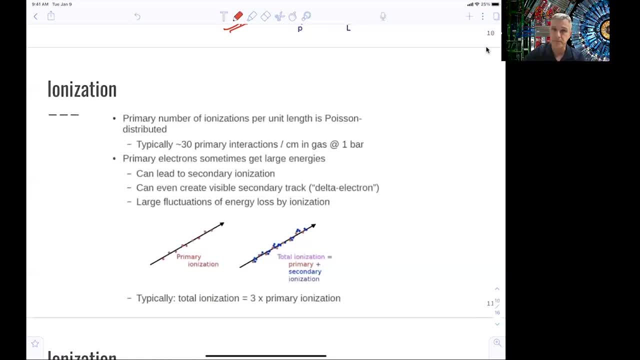 Yeah, Yeah, More in denser material. If you have kicked out an electron in your ionization process, that electron itself can again lead to secondary ionization, And once those electrons reach sufficient energy, it's sometimes visible as individual tracks themselves. 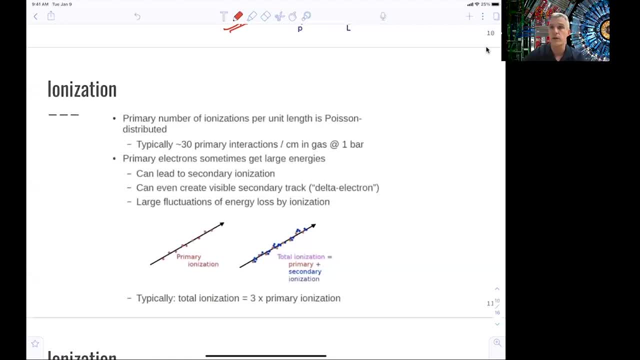 They're called delta electrons, so newer particles which are visible in your tracking detector. Energy fluctuations can be really really large through ionization. Sometimes you have a really tough interaction and you transfer a lot of energy to the electron, while the mean number is well under control. 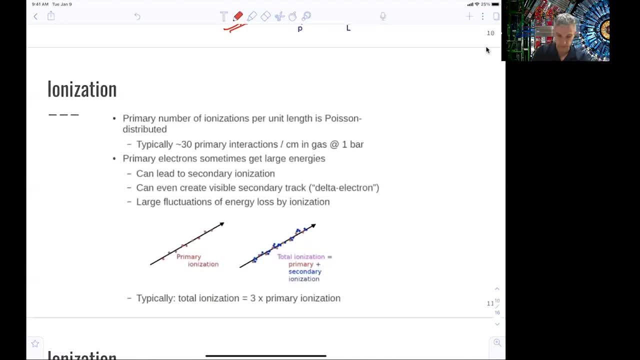 So interesting just to give you a feel again. you have about 30 primary interactions per centimeters in gas. The total ionization energy you find is typically three times the primary ionization energy. So you cause those seeds of ionization and then the energy moves away from this initial track. 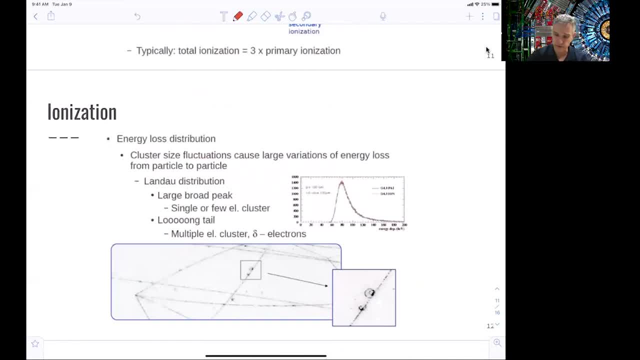 When you look at the energy loss distribution. this is a nice plot here. I made many, many years ago of the energy loss in a piece of silicon of 100 GV pion. So this pion loses its energy primarily through ionization and this is a small piece of silicon which we use here. 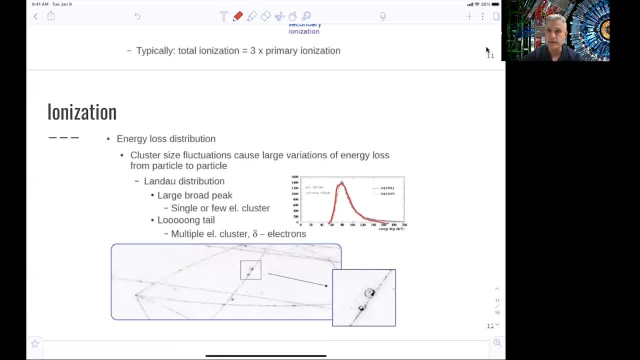 So you see this distribution, typical distribution called the Landau distribution, with the most probable value, and then a very long tail, And this tail here is dominated by those delta electrons I was talking about In bubble chamber or cloud chamber pictures. you see those delta electrons here. 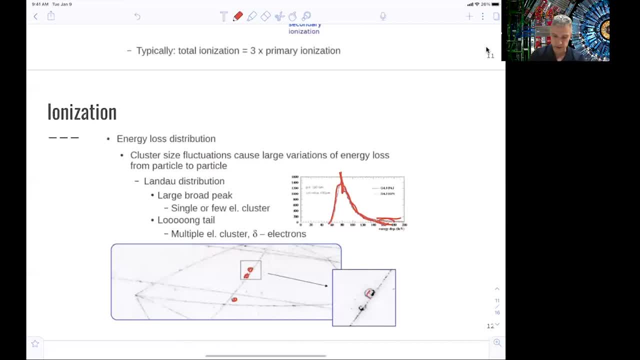 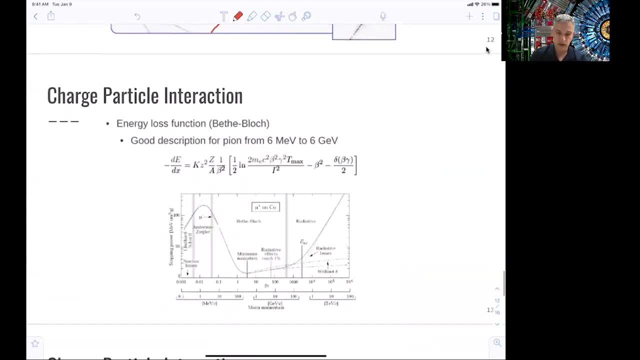 as little curls of ionization along the main part of your particle, leaving ionization track. The energy loss of particles, of charged particles, can be calculated using the beta Bloch formula And it's a very good description in a specific energy range. 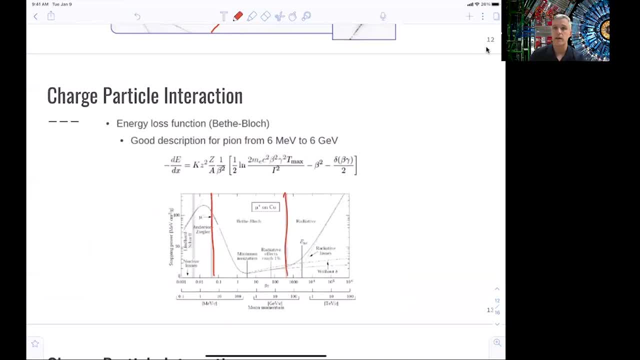 in the energy range which is dominated by ionization, And so the formula is given here. We'll discuss this some more in our recitation section. But you see, here, in this medium energy range, you are dominated by this beta Bloch, This beta Bloch formula, or ionization. 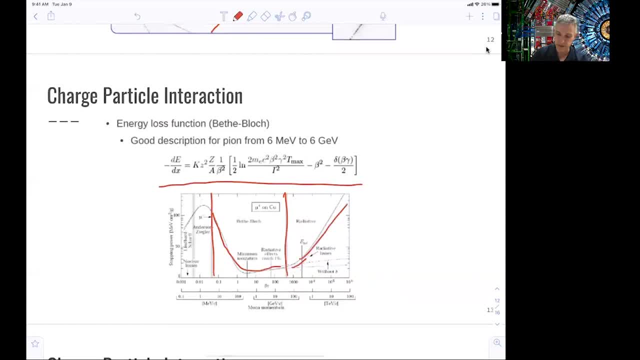 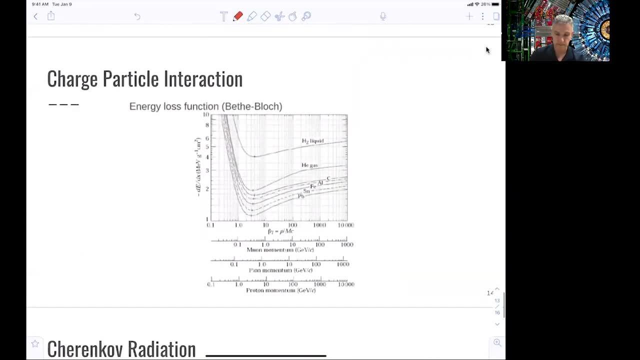 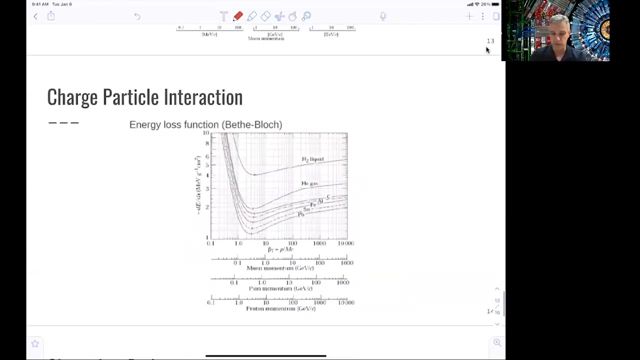 where when you go into higher energies here you find additional energy loss through radiation. So we can study the details of this beta Bloch formula. One interesting point is the particle dependency of the energy loss And you see this here shown for muon, for pion. 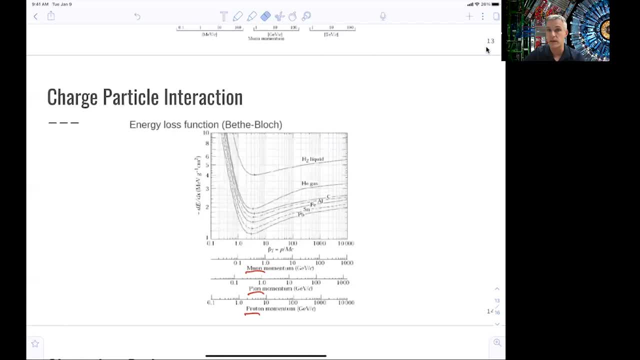 and for proton. If you measure the energy loss of a specific particle in a reasonable momentum range, you can use that information in order to learn which particle was traveled through your detector. So you can use energy loss in some cases in combination with a momentum measurement.